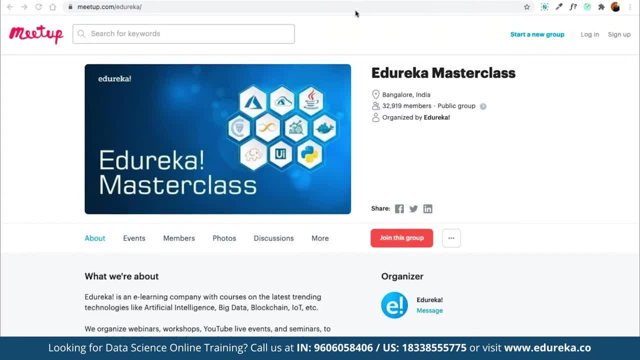 was started back in 2019, and since then, we have been closing into more than 32,000 members so far, And in these masterclasses we have been conducting multiple webinars and live events on different topics, including blogging and other things. So let's get. 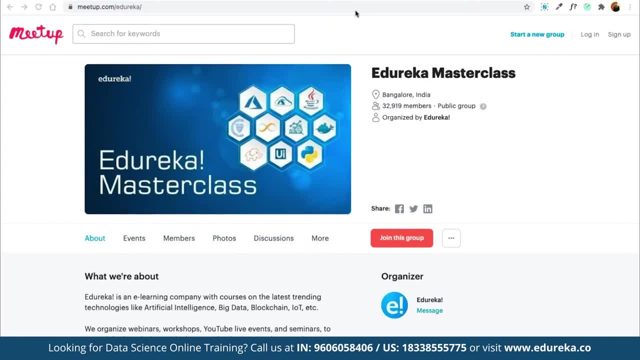 started, So let's get started. So, if we look at the program, you can see here that we're launching a period for you. We have someại for the following masterclasses and this is going toри us to have a brief overview, And the first part is we are going 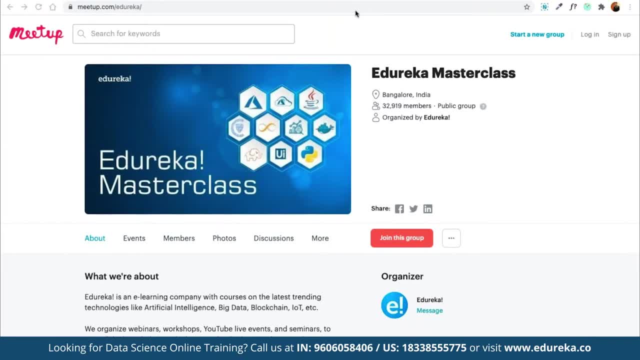 to be talking about core technologies, so learning how toπtun on blockchain, IoTt, artificial intelligence, machine learning, big data and multiple frontend and backend development technologies. Here we are going to start our discussion on SVN as in support. 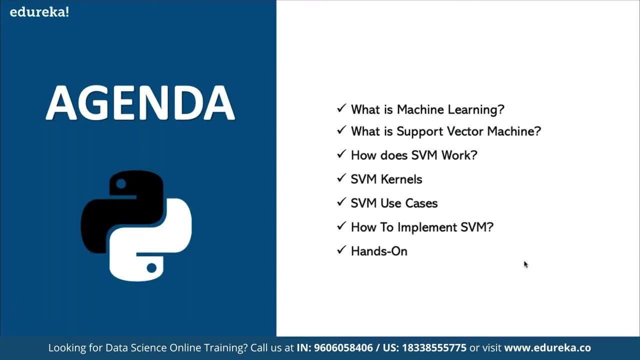 vector machine, How exactly this is structured and how exactly this is going to be helpful for us. So first of all, we are going to talk about what exactly is machine learning- to have a quick clarity on that, And then we are going to talk about what exactly exists. 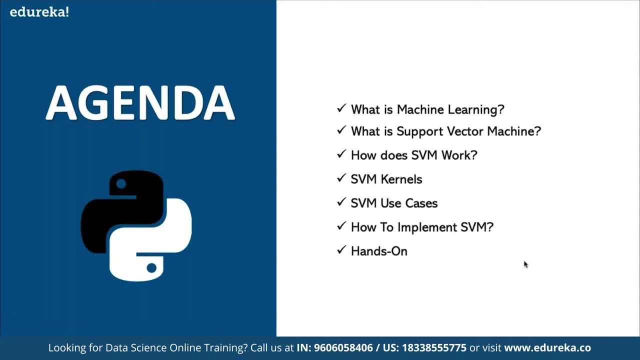 for us. Let's see what exactly we have been talking about with the masterclasses variances: a support vector machine, and then we'll talk about how exactly it works. and then we'll talk about the svm kernels, and then we are going to talk about the components. 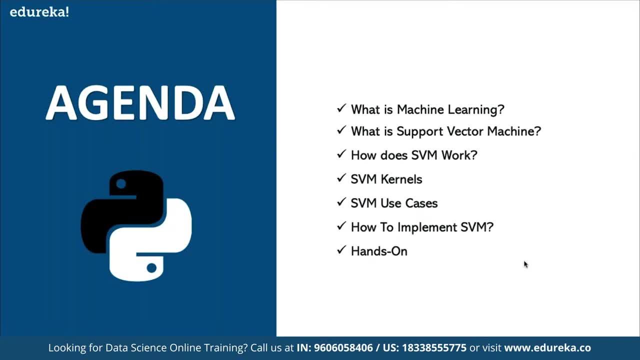 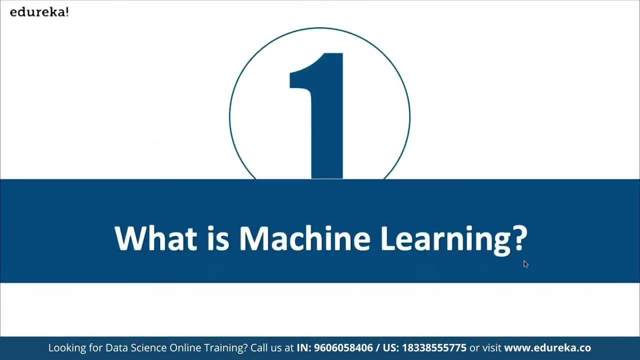 of really that process of implementation of svm as a part of a discussion, and if time allows and we can also see a small hands-on on top of it as well, all right. so first of all, if we talk about machine learning itself, so what exactly is machine learning? so machine learning is simply. 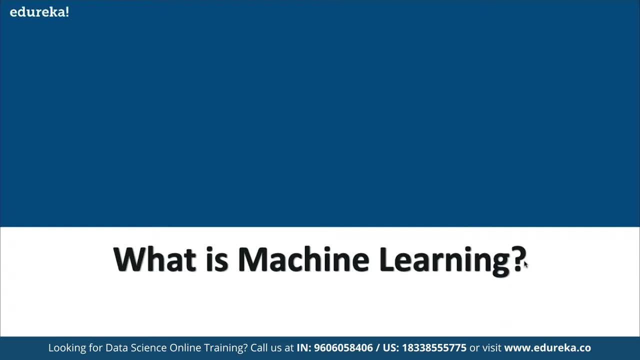 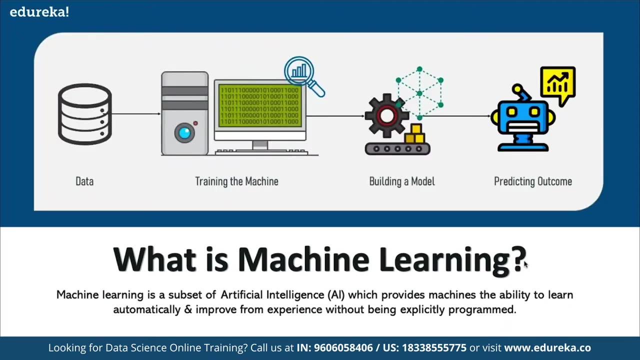 making sure that we are going to automate the entire system by using a good amount of data set right, so we can say machine learning is simply the process of feeding a machine enough data to train and predict a possible outcome using the algorithms which we have the access to. 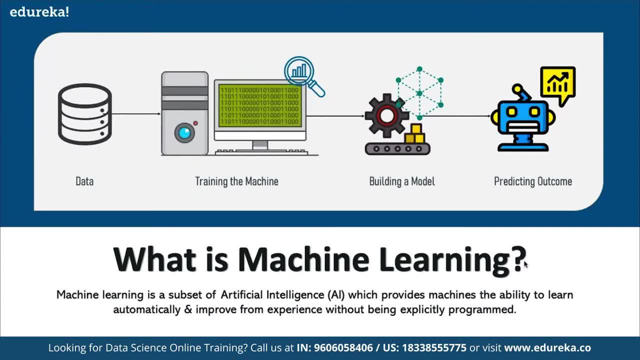 so, basically, if we use more data set and we can increase the accuracy of the results and, let's say, you may have used multiple predictions made in support before any major match, right? so in this case let's take an example for a football penalty session. so the data of previous performances are going to be considered. so let's say, the goalkeeper has 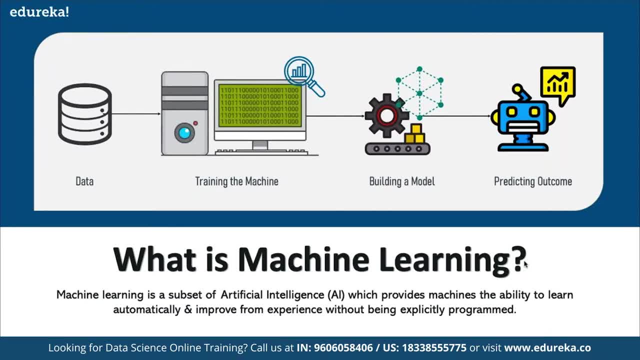 saved all the penalties to his right in the last 50 penalties he has saved. now this data will be crucial to predicting if he or will will save or he will not save the next penalty faces. so there are other factors to consider as well, and another example can be the suggestion that we get while 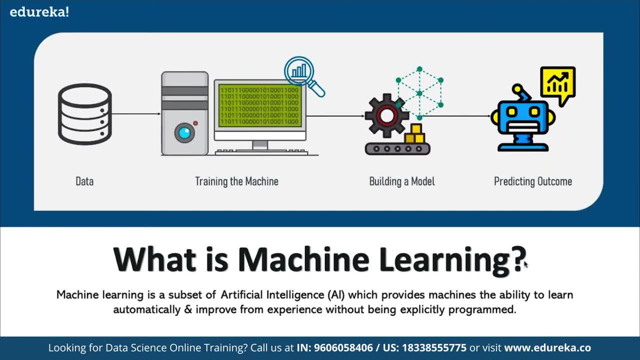 surfing the internet, so the data of our previous choices are processed to give us the most favorable content we are most likely to watch. anyhow, machine learning is just feeding the machine an ample amount of data, the egg. there goes a lot of processes, algorithms and this is of factors to get the optimum results. 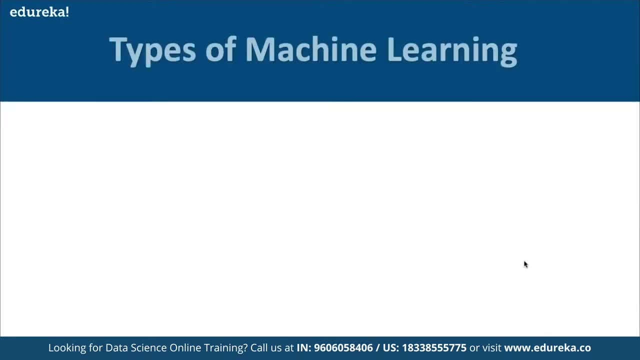 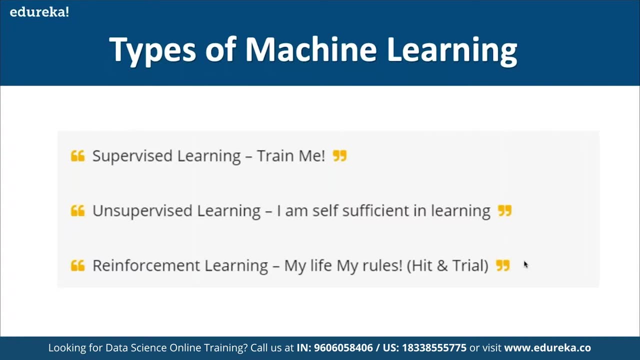 all right. so here, basically, we have three main types of machine learning as well, where we have supervised, unsupervised, and then we have reinforcement learning. so supervising simple dances, train me, it works. on a simple training we have a freedom model. then only it can work. 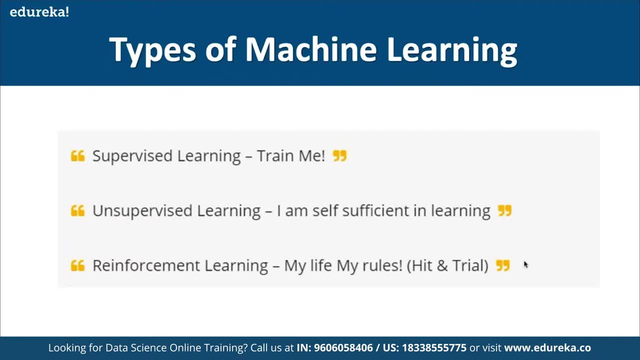 and an unsupervised earning is I'm sufficient. I'm self-sufficient in learning, based on the old learning. we are simply going to allow them to have looking, to allow them to have the access as well. so we are going to allow them to have the access as well. so we are going to allow them to. 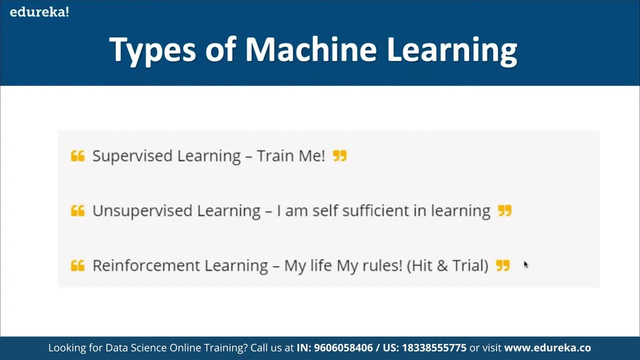 have the access as well. so we are going to allow them to have the access as well. so that is what we are going, so that is what we are going to define. so, based on their own understanding, they are going to work accordingly. that's how it's going to work, and then we are going to work on reinforcement. 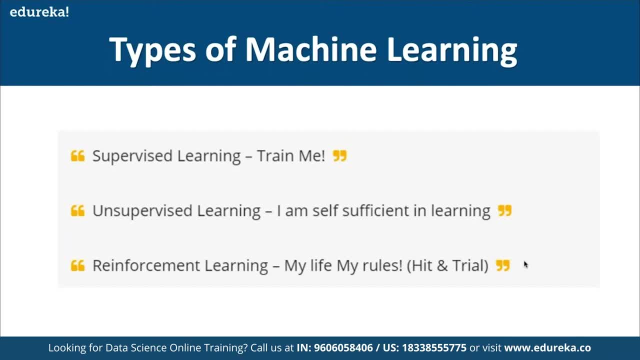 learning. so reinforcement learning is simply learning on its own, based on the feedback. we simply trade, we simply let the system know, okay, if they have done a good job or not, and based on that only, they simply try to get the best product possible output. that's how it works. 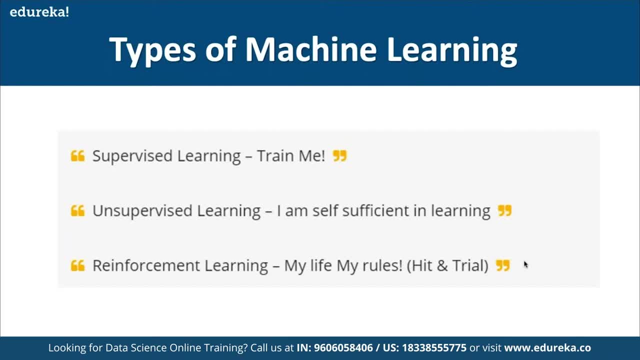 all right. so supervisor and supervisor learning: we use multiple label data set to train the system and under unsupervised learning we use unlabeled data set. so the data is sometimes unlabeled or we can say uncategorized, and the machine makes the best, the best possible reference and predictions without any supervision. and then 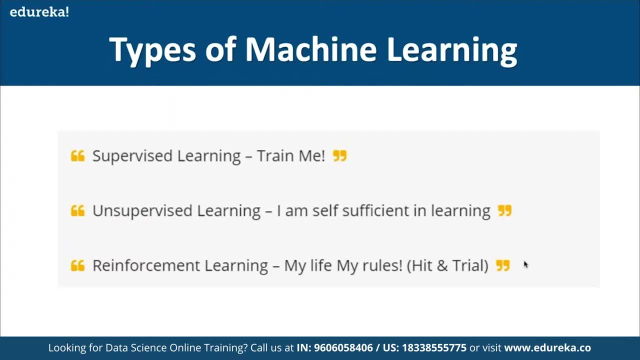 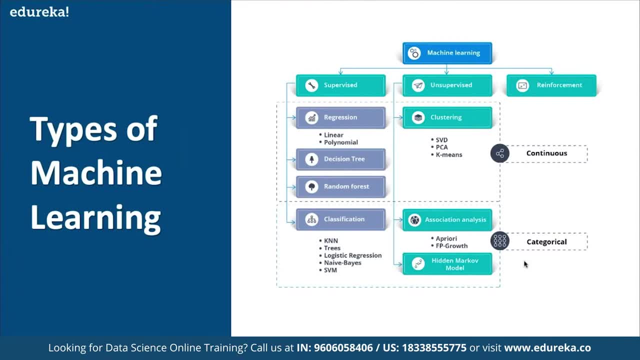 n reinforcement learning here. so that's how we discuss again here. we have supervised, again under supervise we have multiple models, like we have regression decision tree. we have reinforcement models. we have different models currently available, whereas in under unsupervised we have multiple models, like we have clustering. we have 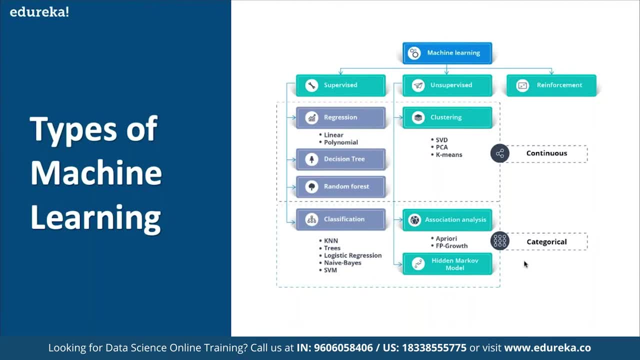 association analysis. we have hidden markup model. so again, the kn crease, largest regression, logistic regression, knife face and svm, they all are types of custom specification where, if we talk about the a priori, if we grow, k means pca, svd, they all are part of unsupervised and, again, reinforcement is simply based on its own structure that we are going to. 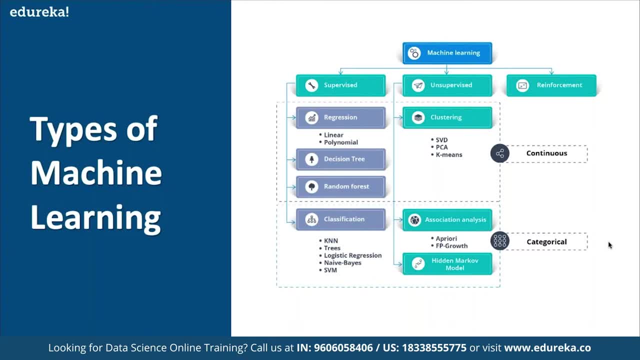 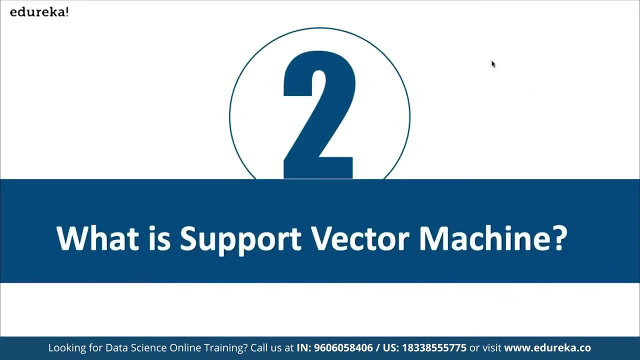 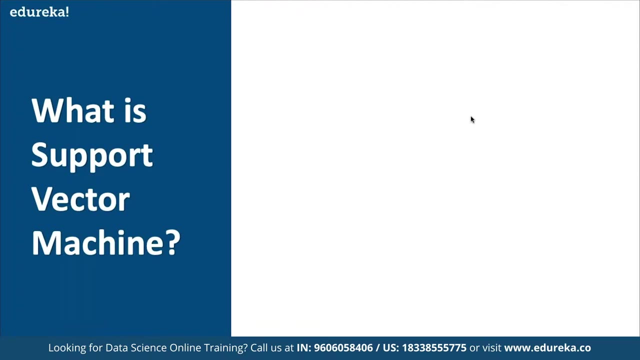 discuss as we proceed further, step by step. all right, so now. next is we are going to discuss on what exactly we mean by support vector machine. so a support vector machine was first introduced in the 1960s and later improvised in 1990s as well, and it has basically a supervised learning machine. 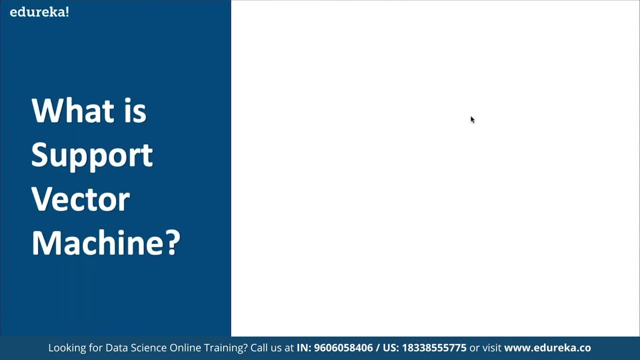 classification algorithm that has become extremely popular nowadays because of its- you can say- efficient results and especially for the complicated scenarios, it can deliver it for us as a part of support vector machine. as you can see again, simply, it is like a discriminative classifier that is formally designed by a 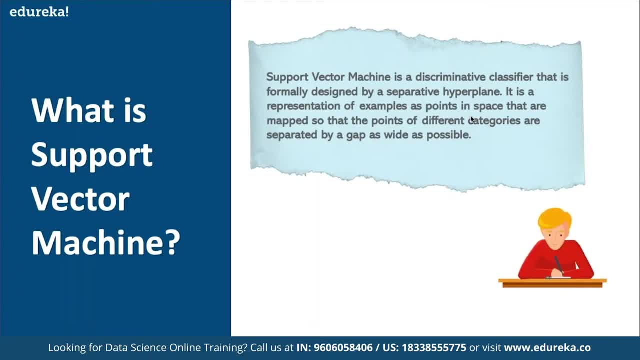 separate hyperplane itself, and svm is implemented in a slightly different way than the other machine learning algorithms, so it is capable of performing classification, regression and outline direction as well, and support vector machine is basically again simply designed by the separative hyperplane instead, as we discussed. so basically here we can have multiple data pointers that can be matched. 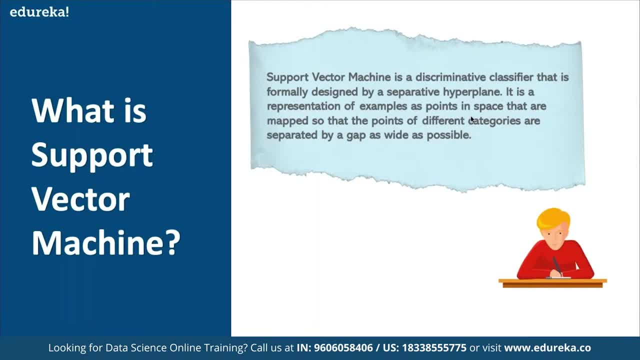 so that the points of different categories are going to be separated by a gap, and, in addition, we can have multiple data points that can be matched, so that the points of different categories are going to be separated by a gap, and, in addition- so basically, svm can also perform non-linear classification. 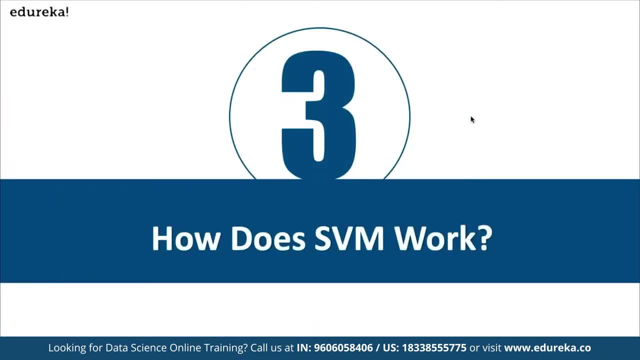 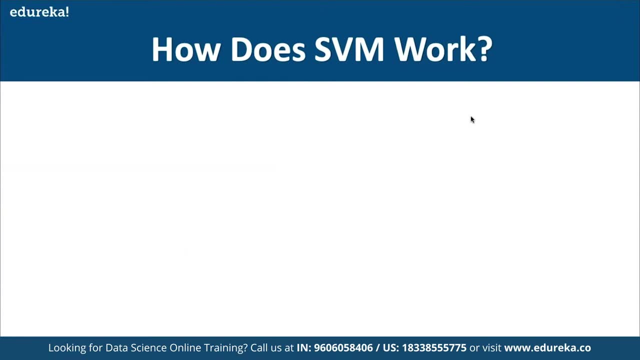 so we'll be talking more about the how exactly support vector machine works as you proceed further. but there are multiple advantages of using svm as well. for example, it is effective in high dimensional spaces. it is effective in cases where the number of dimensions in greater is greater. 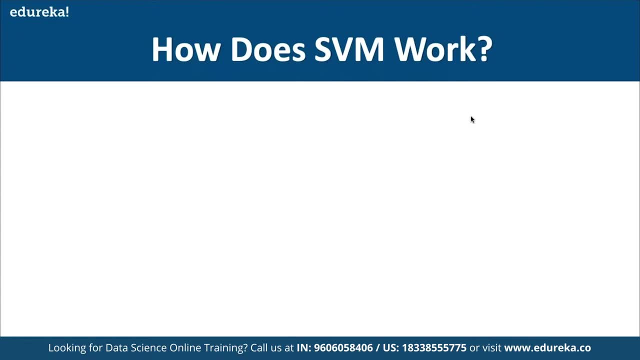 than the number of samples and it is okay. it simply uses a subset of trading points in decision function. that makes it memory efficient and it has different kernel functions that can be specified for discussion function. that also makes it versatile. and same way we also have multiple. we can say downside or we can suggest advantages of using svm as well. so the number of 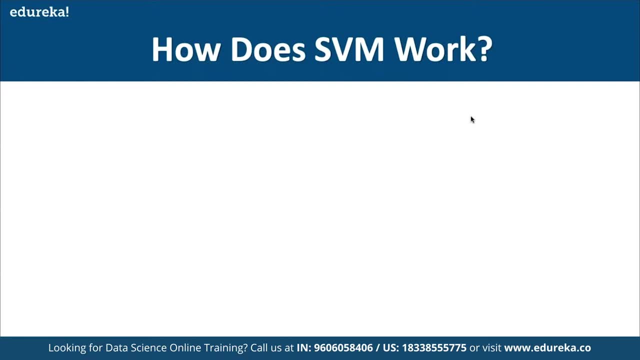 features is much larger than the number of samples, then we can simply avoid overfitting and choosing kernel functions. and again, recognizing them is crucial. and sdm did not directly provide probability estimates and these are calculated using the five fold cross validation. and how does svm work? so the main objective of a support vector machine is to segregate their given data. 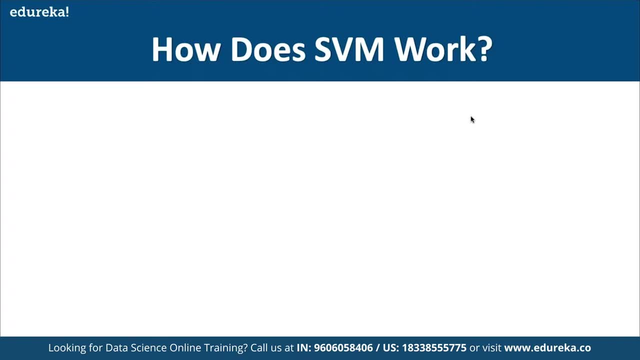 in the best possible way and when the segregation is done, the distance between nearest point is known as the margin, and the approach is set to a hyper, basically hyper- plane with the maximum possible margin in the support vector, as we can see here. that has been right now presented. 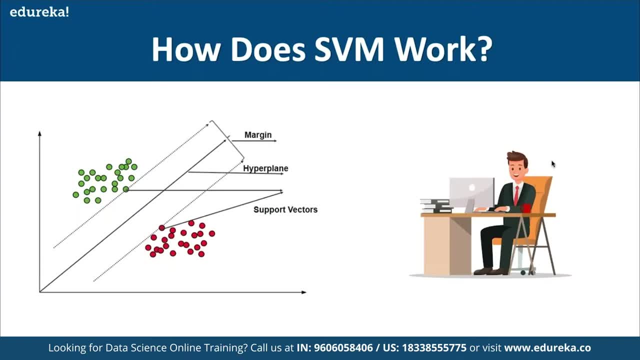 all right, and now basically here to select the maximum hyper plane. so now, in the given sets, the support vector machine follows again. multiple sets, for example, is simply going to generate the hyperplane which segregates the classic classes in the best possible way, and then we are going to select the right hyperplane with. 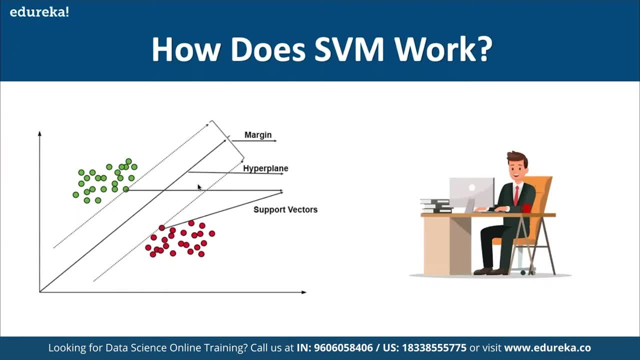 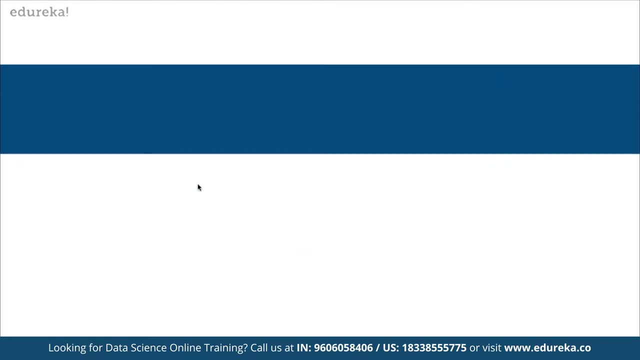 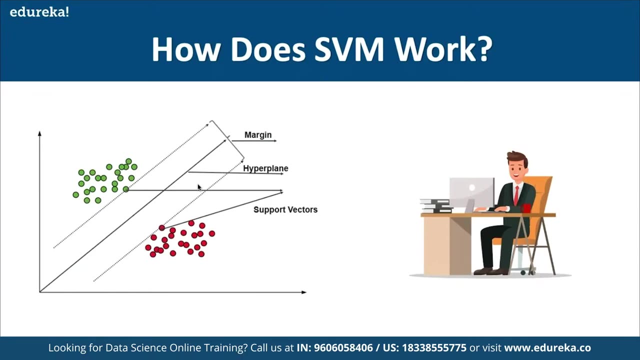 the maximum segregation from either nearest data pointers. so basically there are different ways of or even dealing with inseparable or, we can say, non-linear planes as well. so, for example, in some cases hyperplanes cannot be very efficient and in those cases the support vector machine uses. 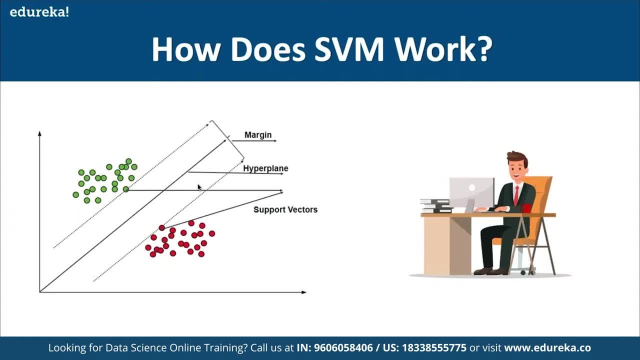 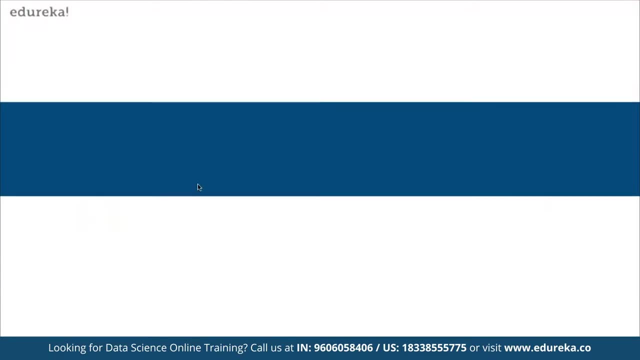 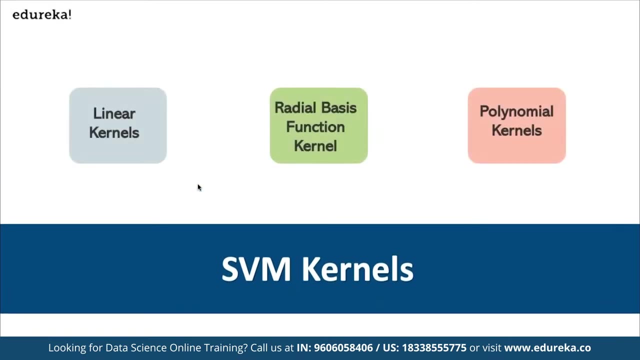 a kernel tick from a kernel trick to transform the input into a higher dimensional space, and with this it becomes easier to segregate the pointers. so now let's talk about the svm kernels. so basically, svm kernel adds more dimension to a lower dimensional space to make it 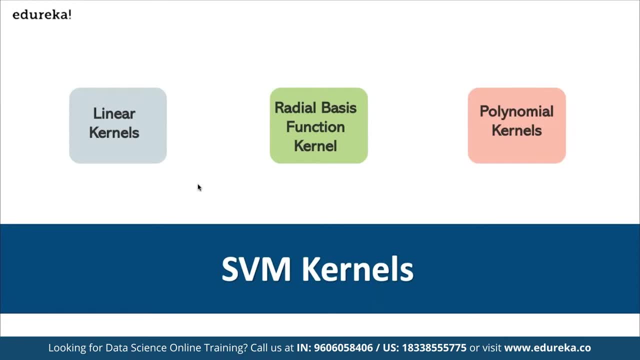 easier to segregate the data. it converts the inseparable problem to separable problems by adding more dimensions using the kernel trick. and the support vector machine is implemented in practice by a kernel and the kernel trick helps to make more accurate classifier. so we can take a look at different kernels in a support vector machine. like we have linear, we have radial. 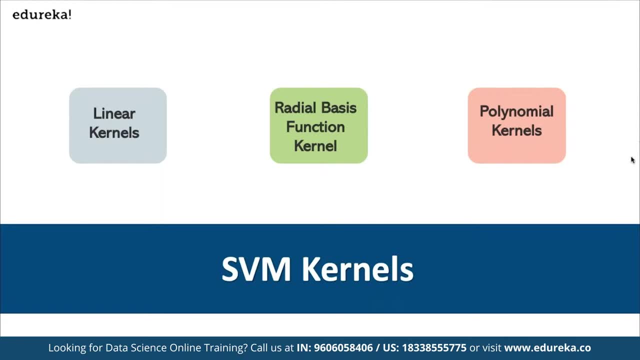 base, and then we have polynomial kernels as well. first of all let's talk about the linear kernels. so a linear kernel can be used to as a normal dot product between any two given observations. so the product between the two vectors is the sum of multiplication of each pair of input values. so 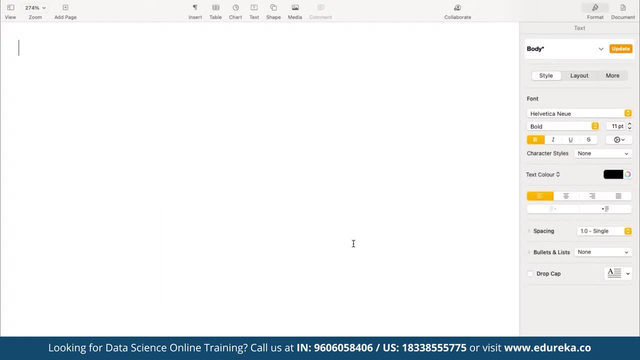 we can understand this right. so if we talk about the linear kernel, so if you talk about the linear kernel, so basically, as we as we discussed, linear color can be used as normal dot product between any two given observations. for example, here we can define this one as opposed to zero and it can be added to. 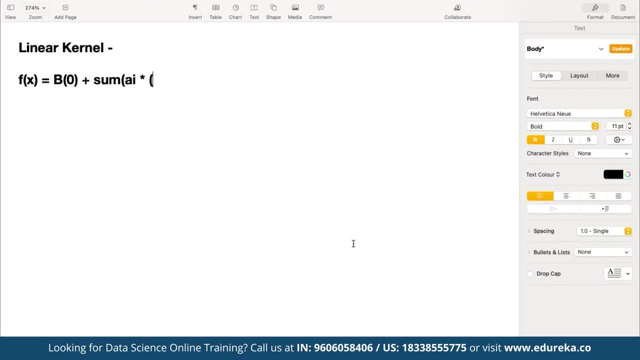 sum of, let's suppose, multiplied by x, xi, all right, going to be. the product between two vectors is the sum of multiplication of each pair of input values as a part of simple linear kernel equation. and then we have polynomial, so this one is for linear. then we have our polynomial kernel, so polynomial kernel is what polynomial kernel is. 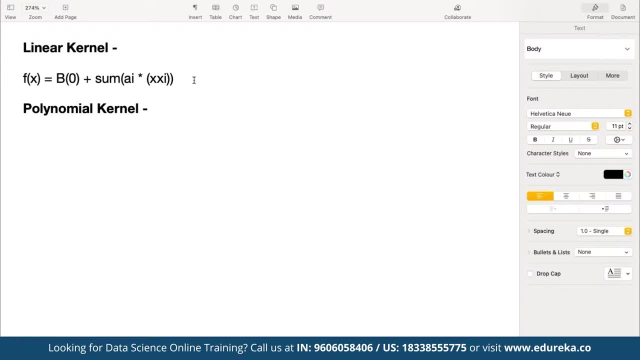 like a. it's rather generalized form of the linear control, and again it can distinguish curved or non-linear input space. so for example, here we can refer this as opposed as k, and then we can define multiple pointers, i suppose x1, x2, and then we can simply add this to a plus now here: 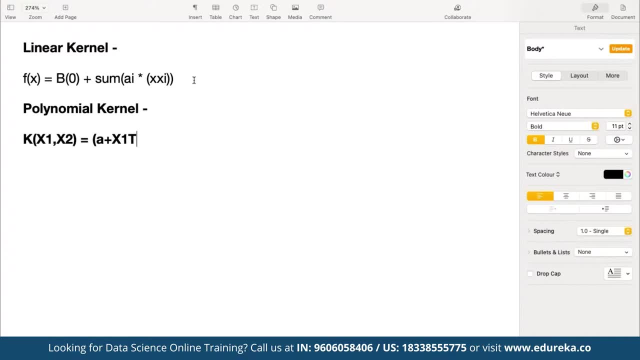 we have defined, suppose, x1, and again all of the click will be defined here: x1, t and then x1, for again this value for x2, here for x2, and again the entire one has to be raised to power b itself. so next we, after polynomial, we are going to have, we also have radius space. so here: 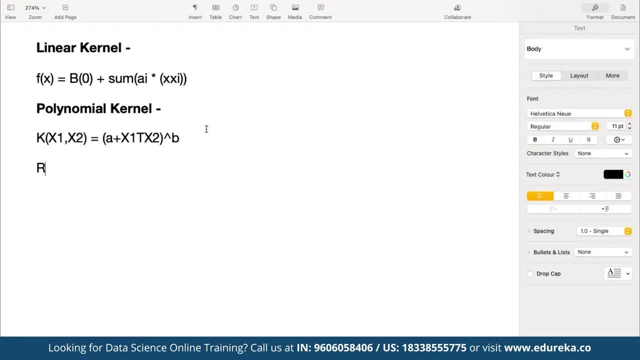 after polynomial we have the radial basis function kernel. so in terms of radial basis function kernel. so here the radial basis function kernel is commonly used in the svm classification and it can be turned into a dimension of x and x. so a constructor is repeated between a as y, and then we can define this for x1 minus. this is going to be x2, and then it has to. 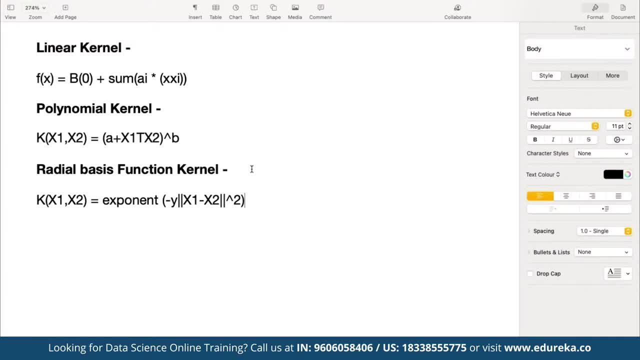 be raised to power 2. so basically, x1 minus x2 is simply going to be the euclidean distance between the x1 and x2. so we can say: x1 minus x2 is euclidean distance, is the euclidean distance between x1 and x2, here and where? if we talk about here, if we talk about the 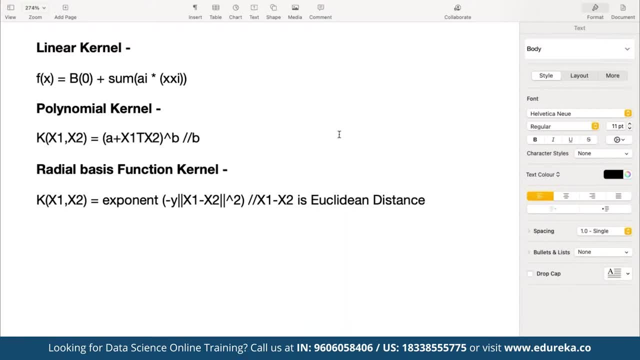 current component for b. so here we can say b is what b is, b is the degree of kernel in case you don't have, in case you don't have the knowledge of of it yet, and then a is going to be. or we can say a is what a is the constant term, a is the constant term that we have. 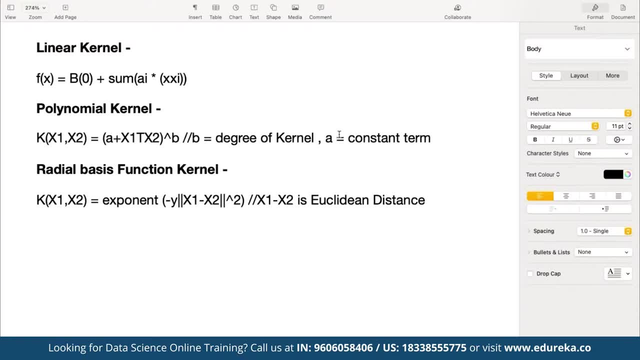 so here we have linear polynomial and then we have radial basis function, so there are multiple use cases. so before we proceed further, so there are multiple use cases of the serial base conver- i can say component as well, so here we can use it for the phase direction. 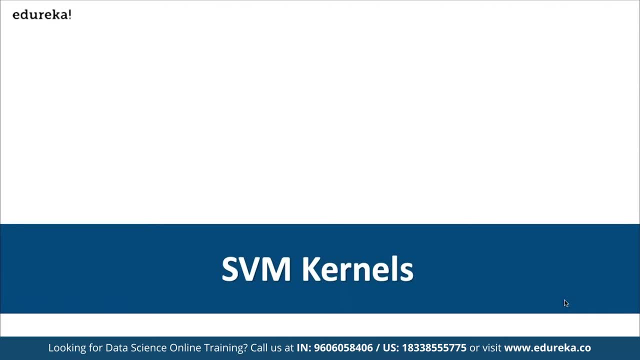 for text and hypertext categorization here. we use it for the classification of images, for bioinformatics, for protein fold and remote homology detection as well. we can use it for different use cases and we can also use for, again, having a prediction control as well, as we discuss in svm. so there, 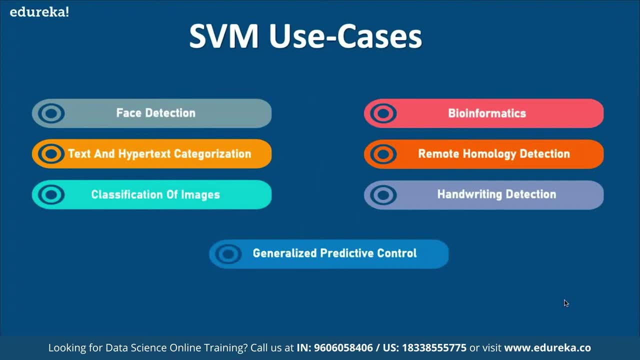 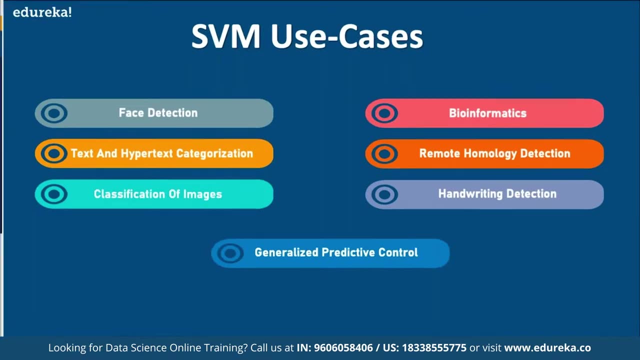 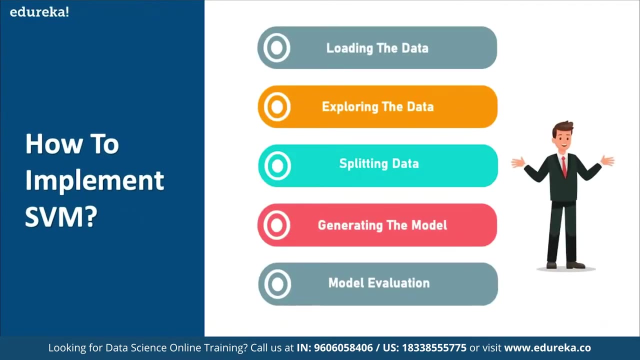 are multiple use cases for face detection, for bioinformatics, for text and hypertext categorization, for remote homology. so these are different use cases that currently available here. so now in terms of how to implement svm. so first of all, we have to load the data, we have to 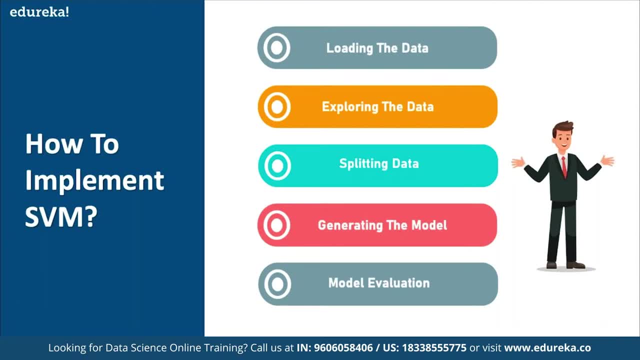 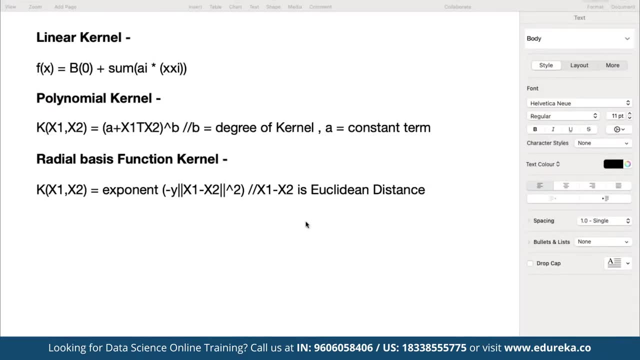 explore the data. we have to split the data, and then we also have to generate the model, and then we have to evaluate the model as well, as we have discussed again, in case we have been confused. so linear is simply going to be the dot product between the 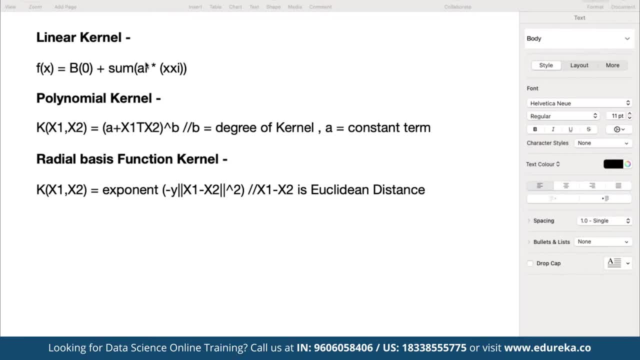 any two given observations itself, and here we define two. here the product is going to be between two different vectors, it's simply going to be the sum of multiplication of each pair, and then under polynomial. so basically here we can distinguish curved or non-linear input space where we have 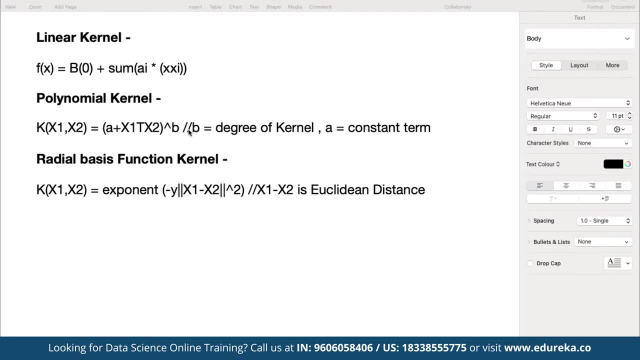 defined the k1 as x1, x2 for where a is where a is simply going to be a constant term and b the power to which we have increases. so b is simply going to be the degree of penalty we are going to make use of, and then, under radial basis, as we discussed. it is commonly used in classification. 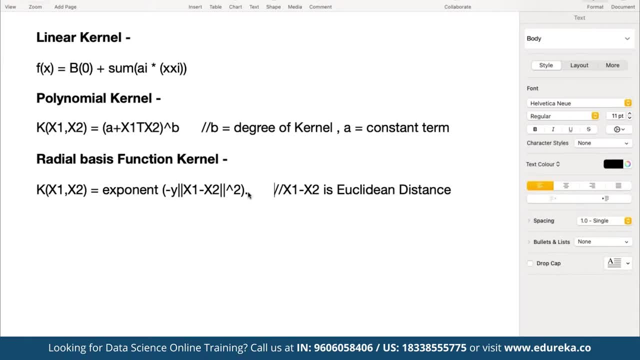 and can map the space in infinite dimensions as well, where x1 minus x2 is simply going to be the euclidean distance, and we can say this one that we define here: x1 minus x2 here is simply going to be the euclidean distance here. all right. so let's do one thing: let's open up pycharm. 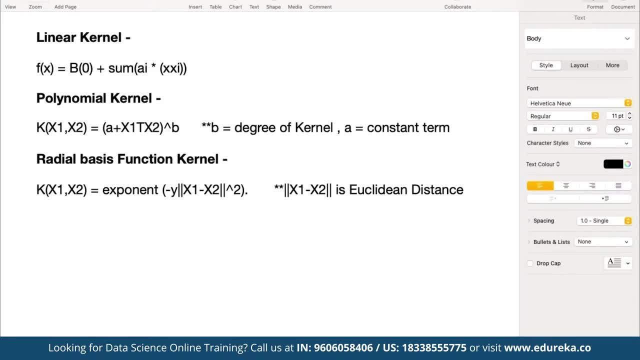 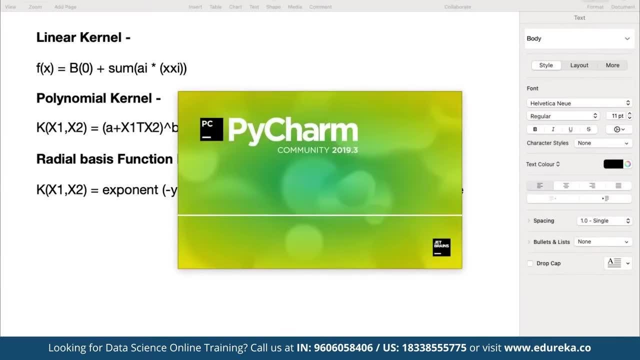 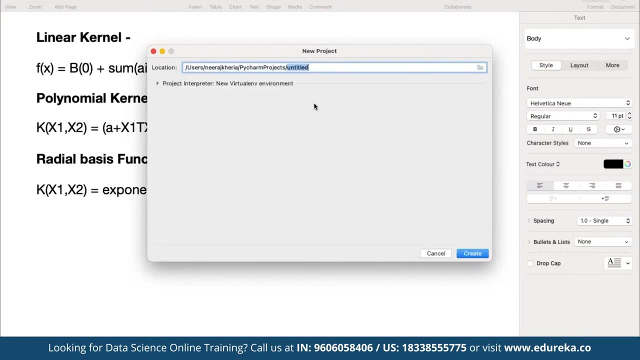 community here. so we can start by simply loading the data set and then working on top of it. so we can use any id. we can use any python id to get started. we can use anything. so let's do one thing. let's create a new project. let's say we name it as svm. 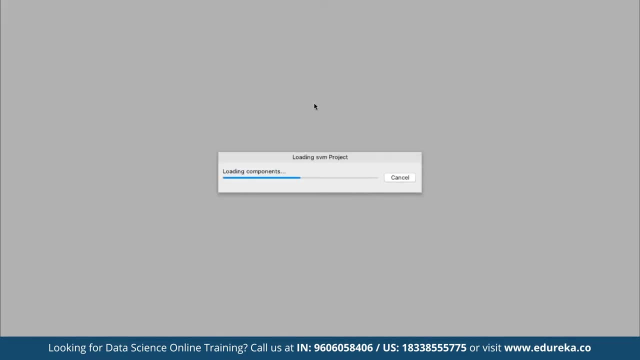 as of now. so in case you don't have the access to svm as of now, so you can go ahead and download the community version. so this is going to give you the access to pycharm, or we can use any other id as well, if required. all right, so here, once we have the project here, we can simply go. 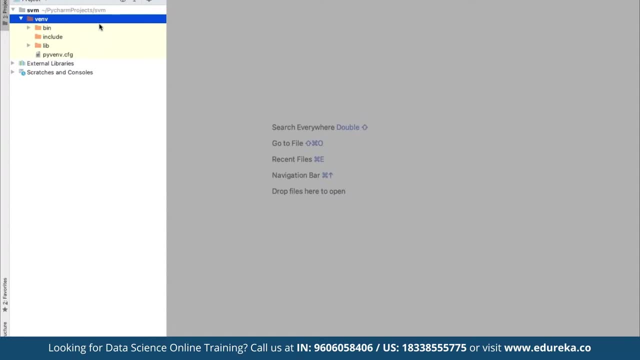 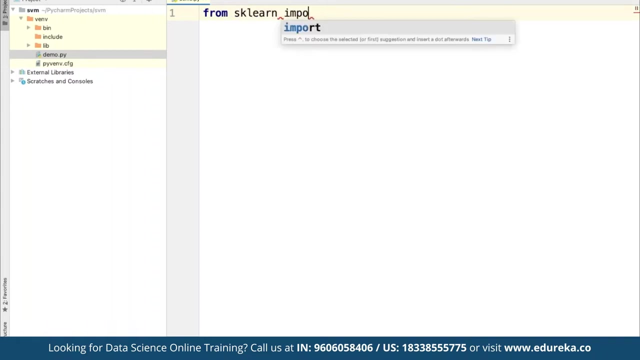 ahead and create a new file altogether, so let's name it as our demo file. so first of all, we are going to work from the skl library, so here we can use from skl. we are going to import the data set, so they they are some sample data set available under skl library itself, so here we can define. 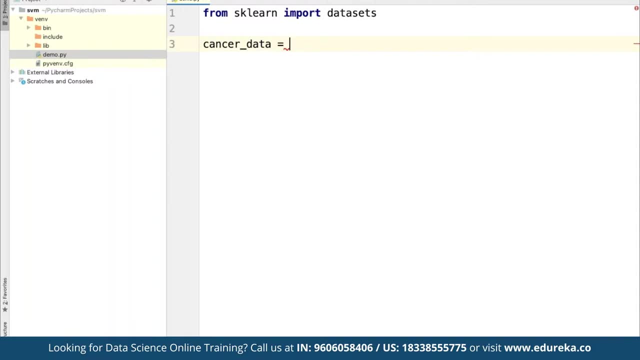 the cancer data set already available under skl and here we can use data set start load and then we are simply going to load. suppose, for breast cancer, we can load this current data set already available and now, if you want to simply print the current data set, that is that we have currently imported. so here we can find cancer. 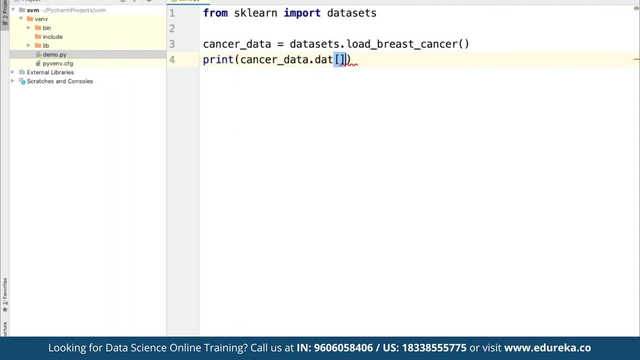 data, dot data. and again, we only want to print the five first rows available in that. so here we can define these statements here. so we have. we are going to use a sample data set currently available and whenever we are going to work on any project, in case they are. 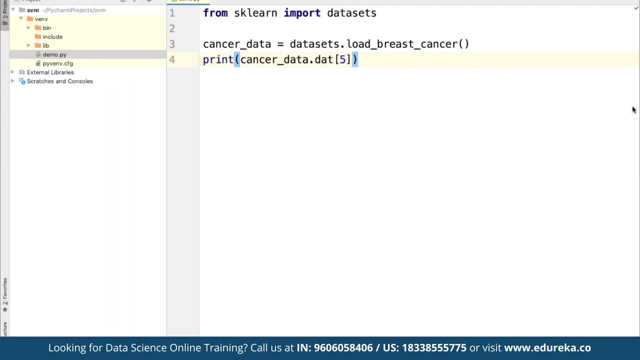 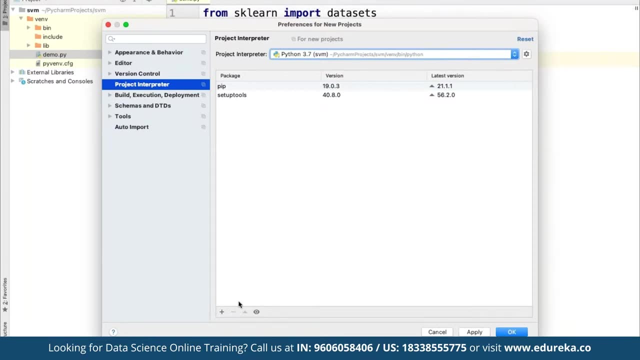 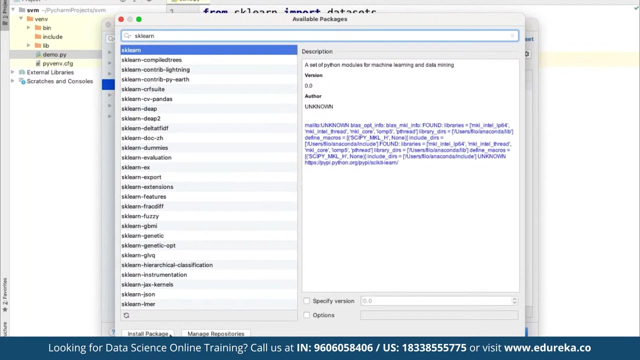 now, in case the data set is not available, then we can go ahead and simply install more libraries by simply choosing the current data set and then here we can go ahead and click on add and from here we can search for any library. that is that we may that may be missing, for example. here we are going. 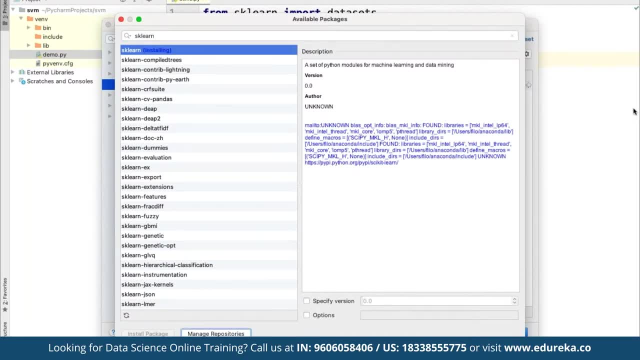 to work on sklan, so we have to make sure that we do import skl, because without skl library we will not be able to work on the svm here. so here we are simply going to work on the sample data set. all right, so, as you can see, now sklan has been installed. so again, this is a. this is a package. 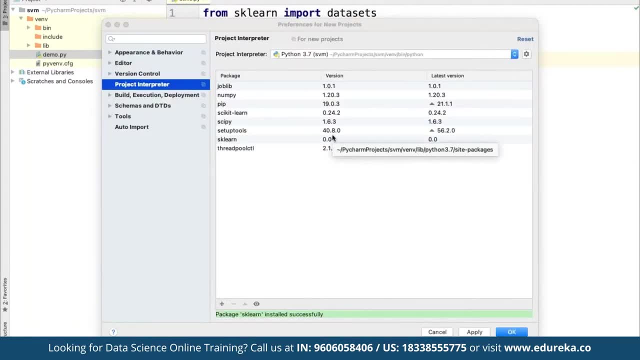 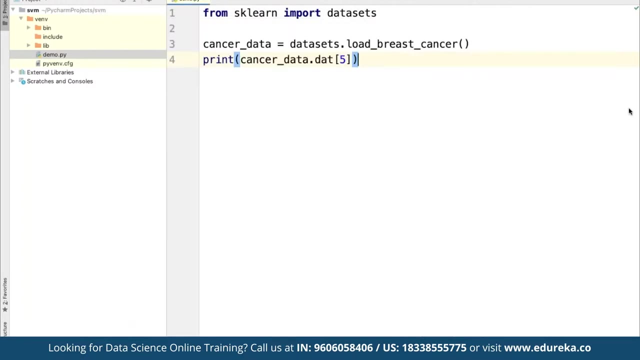 that we are going to work with. so here we can close it now. if we want to work on the other components, we can search for any library and then we can have it installed. all right, so now we can click on apply and then once we now, because if we don't have the library installed, and then if we try to run, 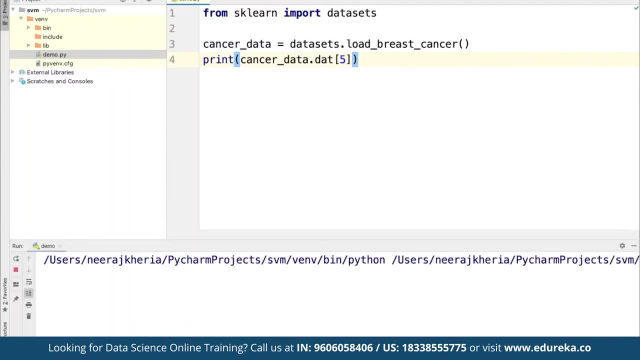 this up, it will simply go to throw us an error and, as you can see, currently this is going to update the package and then from there it is simply going to load the breast cancer register, which is available as an inbuilt sample in sklan. so it is simply going to get connected to the server and then. 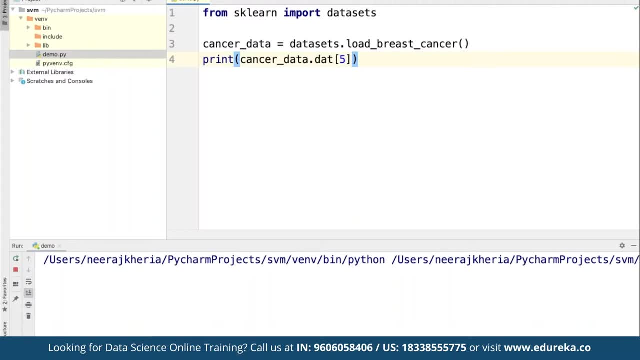 from there. it is going to be going to pull the load, the breast cancer leader set- and then it will simply go to print the first five rows from that data set. so it may take a while, depending upon how, which data set we have imported. so before we perform any calculation, let me just show you. 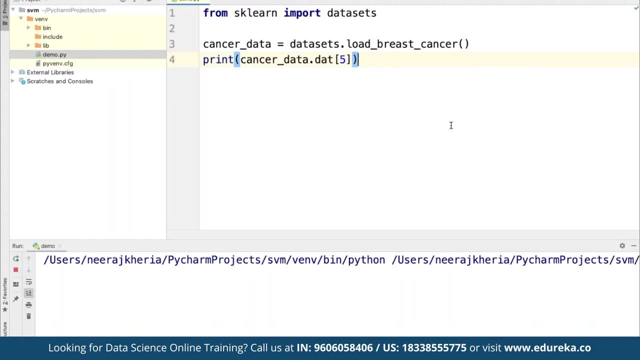 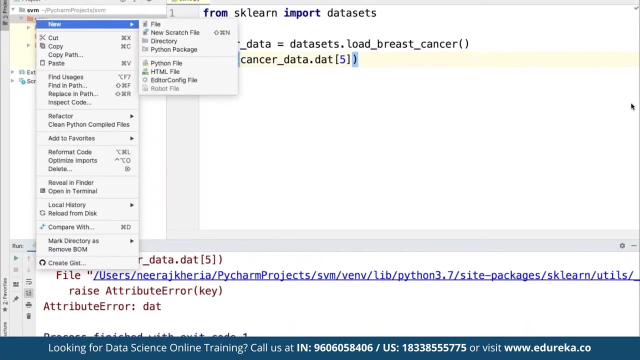 how started this looks like again. in the meantime, this is getting pulled here so we can simply go and create a new file. it has been timed out because of memory error. okay, we defined, we misspelled data. it has to be data itself then only, it is simply going to. 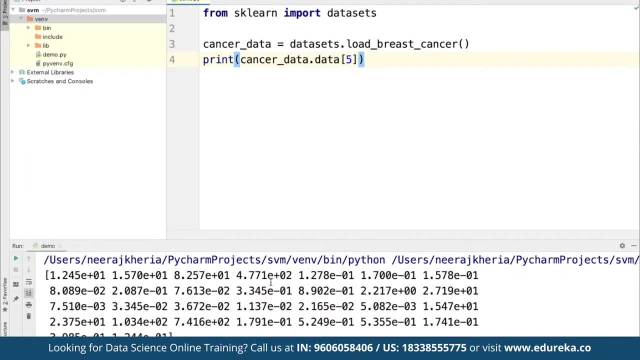 fetch from there. so, as you can see here, now we have the first five rows in terms of this breast cancer data, which has been pulled automatically from sklan, as you can see here right. so now we are going to here. we have defined the data set, right. so now, if we are going to simply, 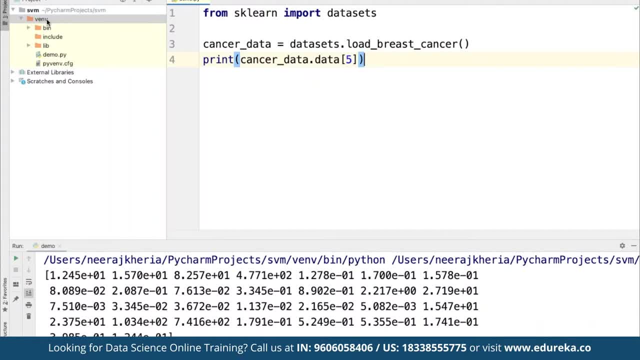 split the data right. so we are simply going to divide the data into training set and the test set to get accurate results, and after this we will split the data using the train test split function. so here we are going to need three parameters, like in the example that we have that we are. 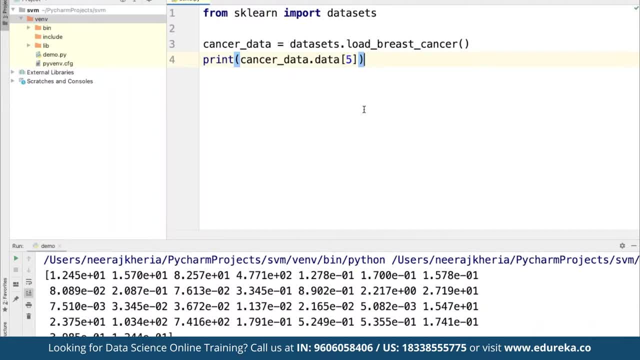 going to see. so from here we are going to load the current data set. so for example now here, now just to over confusion for yours, so we can create a new file. let's say we define since, as suppose number two. so here we can define from sklen. so first of all we define from sklein library, from sklearn. 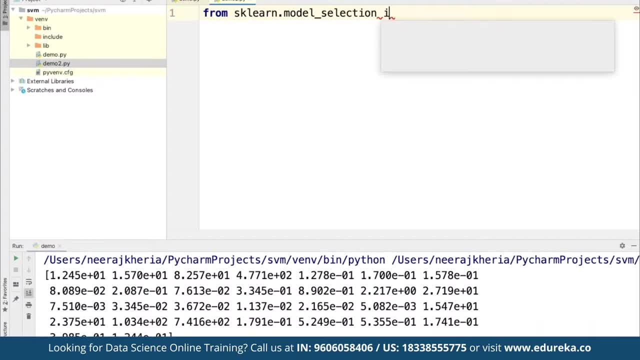 and here we can define model selection. so here we are going to import train test split, as we discussed. we are going to split it and then we will get to find讓 we are going to combine the training solution to learnelet set end, analyze it, to implement side test. to find your data set: here we are going to need three parameters. 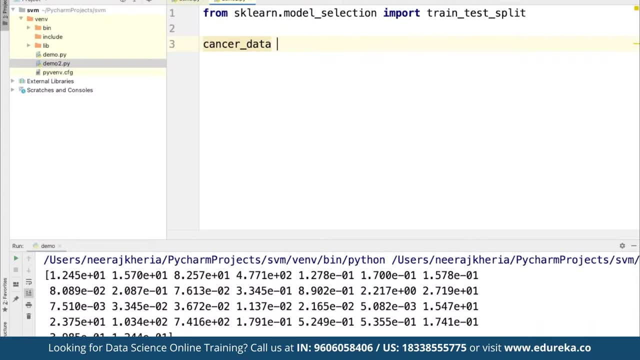 so here we are going to import train test split, as we discussed. we are going to split it and then we can define from sklearn find, from cancer data that we are going to import. so here we are going to find data set dot load rest cancer, which is already available, and then we are simply going to define the models in terms. 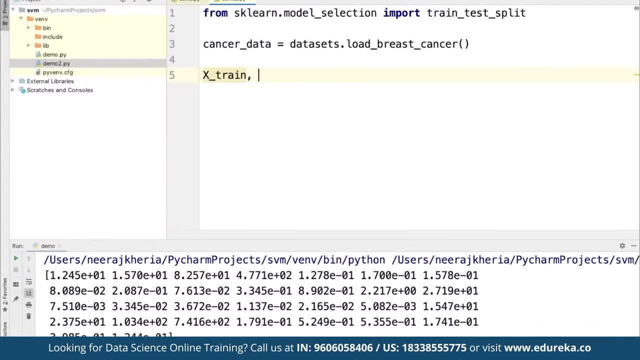 of suppose, here we define x train and then we can find x split. uh, we can define for x test and then we can define same thing for y train, for y test, extreme x test, y train, y test. so here we are going to define this from the same train test split that we are going to import, and then here we 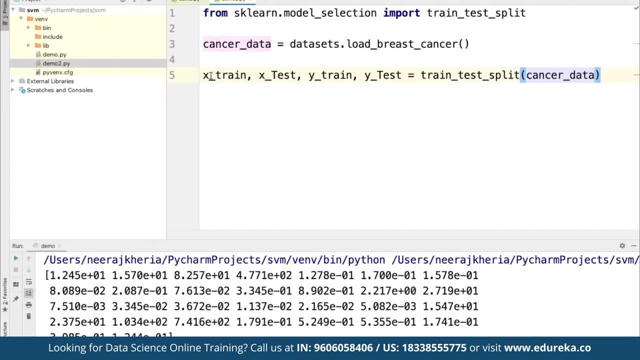 are going to divide them under, from the cancer data and the data which has been imported here, and then we are going to define this for cancer data target. so say, here we can define this for cancer data dot target, and then we can define the test size. here we can define the test size, suppose we want to. 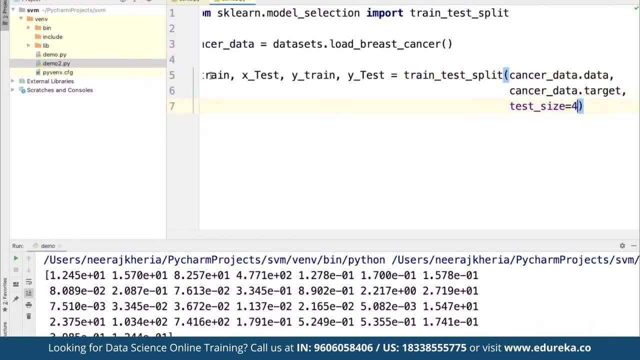 keep the test size, suppose as four, this test has s4, and then we're gonna find random state. we can define random state and suppose, but on anything that we want to have. so here we are simply going to split the data set with the given in the extreme x or x test and the y. 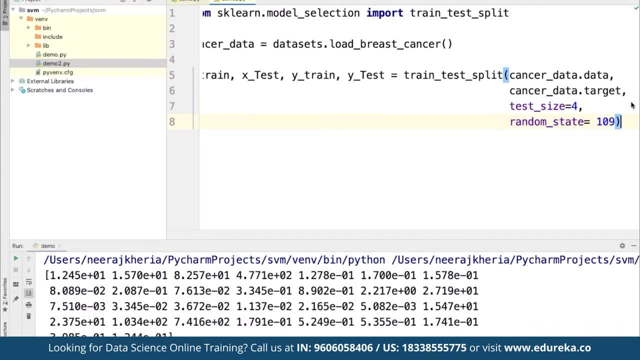 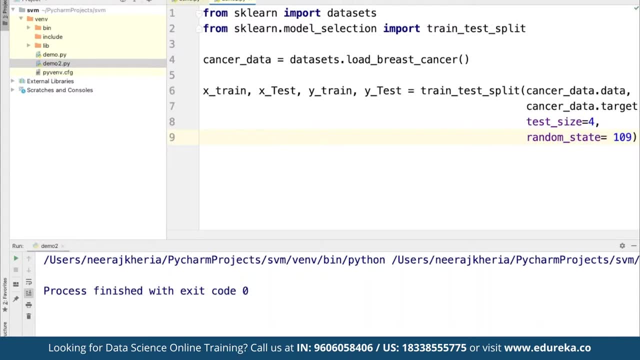 trait and y test here. so here the entire set is simply going to be split. so, as you can see, now that we have split the entire data set, so now we are going to generate the model as well. so what we can do. so now, here we are going to gen, we can say: generate the model and 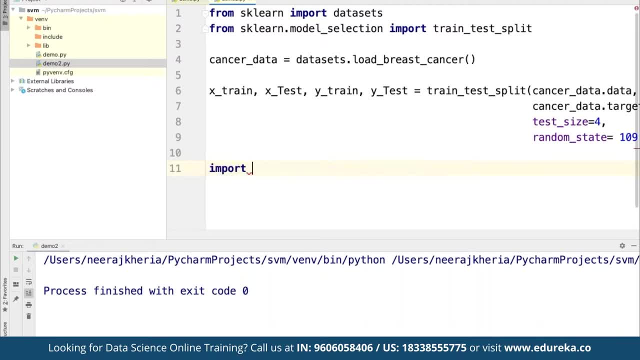 for that we can import. on the library, for example. here we can import, let's say, sk learn, and here from escalon we are going to import the svm. so here we are going to create the library. so here we could create a classifier here. so first of all we're going to find classifier, as suppose. 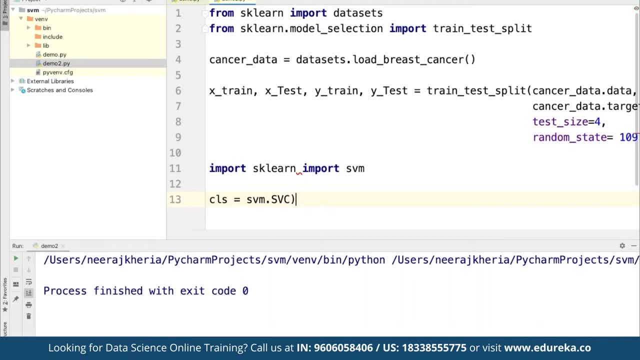 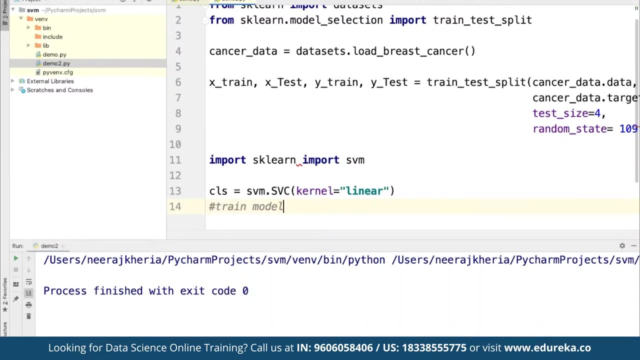 svm, dot svc, and here we can find the kernel. here we can find the kernel as suppose linear, and here we can find the kernel as suppose linear, whatever we want to use, we can define that and then we are going to train the model. so we can say: we are simply going to now train model, so here 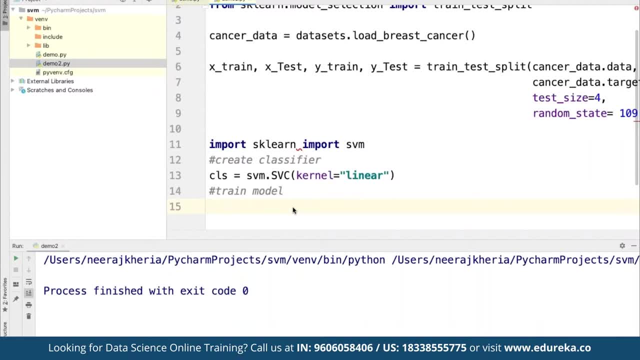 we have create classifier and now we are going to train the model. so for training one, we can define class dot fit, and then we can define this value as x train that we have already imported, and then we can define for y train that have we have already performed the split on. 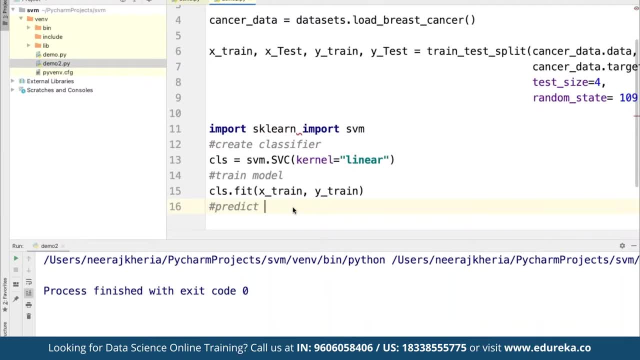 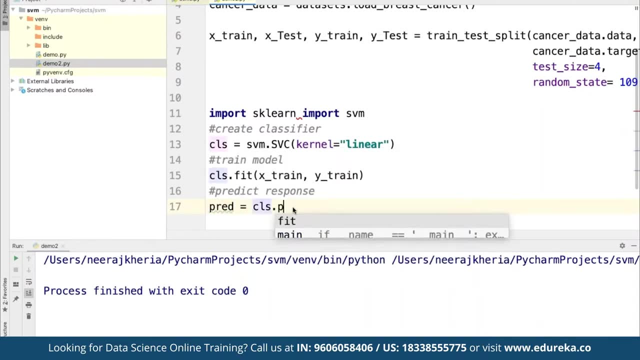 and then, simply, we are going to have a prediction done. so here we can define predict response, and for getting the response we can define prediction as class dot, predict. and for this we are going to make use of x test that we have already defined. we have defined for x train and for y train. and then 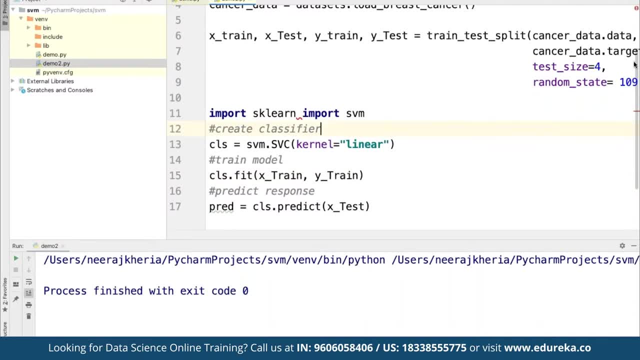 for prediction. we are simply going to do that on the text on the x underscore test that we already have defined. so we are going to do that on the text on the x underscore test that we already have, and then we are going to define the type of data that we have. so that totally depends upon the type of data we 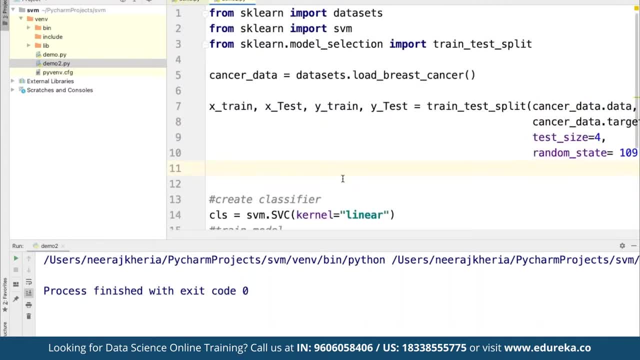 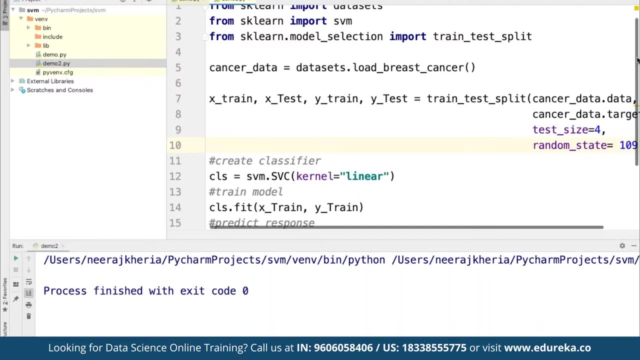 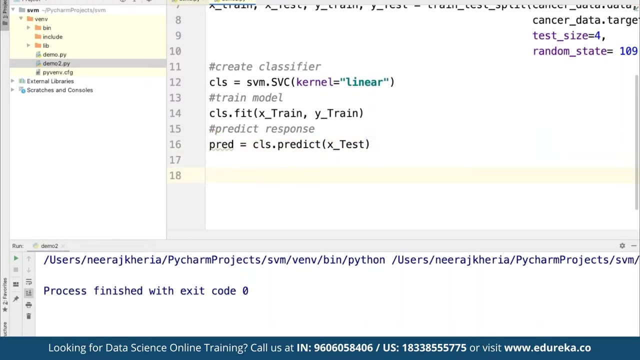 are going to simply import, and let's move this import from the end up here. so you have to define this in the top section from sql and we are simply going to import the svm if we had to find, all right, and now we have to find the classifier. now we are going to evaluate the model and for evaluating the 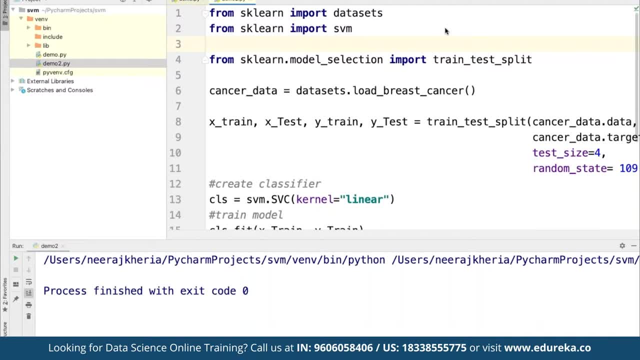 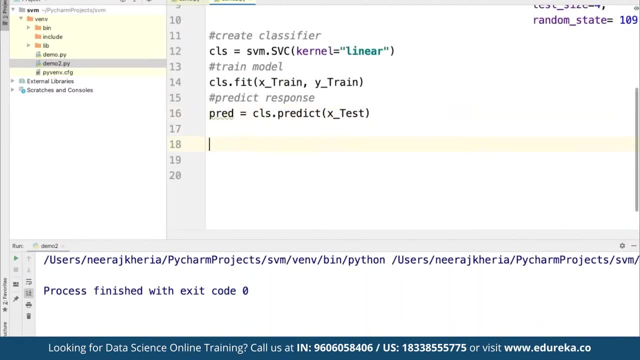 model. we can simply go ahead and define. we can also import other components as well. from sqlm. we are also going to import metrics. so here we are also going to import metric and by using macro accuracy, metric for getting the accuracy we can find, for getting the accuracy we are going to define, we are simply going to print. 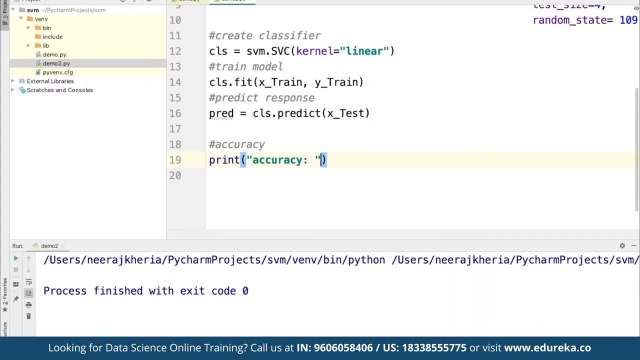 the accuracy of the prediction here, and for accuracy, we are simply going to define metrics, which is again available under the matrix that will, uh, here we have accuracy score and then from here, we are simply going to find y test and we are going to find this one for. 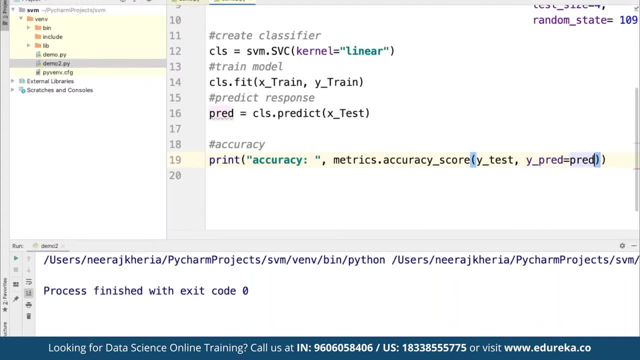 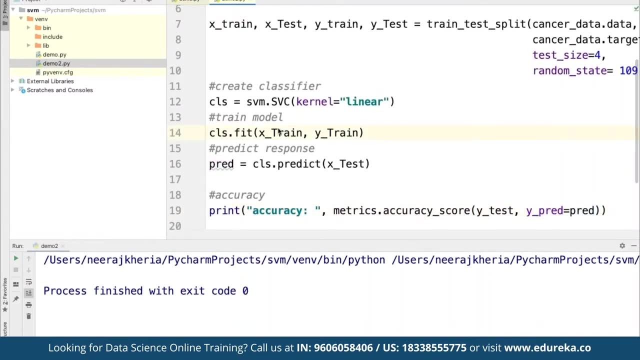 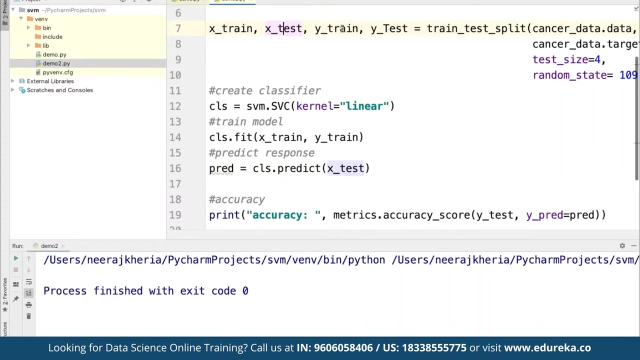 y prediction as well, that we have defined. so i think we have used y test, we have used upper case for, for we have used let's do one thing, let's use small case for everything, just to avoid confusion. let's find this test, train and test again, so you have your y test and then you depend here we define. 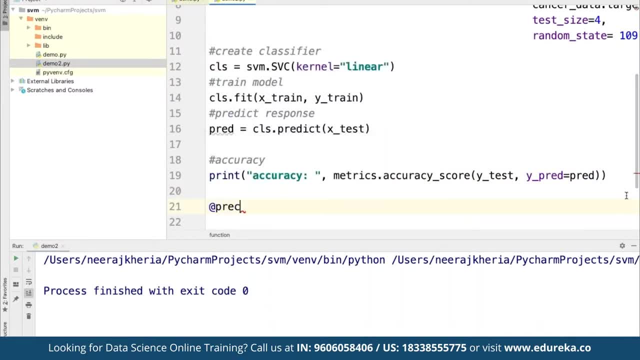 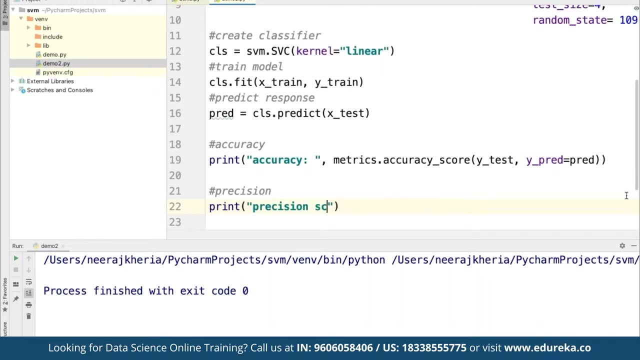 the precision score. and then we get the precision score, um, we can just print it, we can also write it as precision score. and then for finding the precision score, for finding position, we can simply print another statement as precision score. and in here we can again make use of metrics, and for metrics we can define the precision. 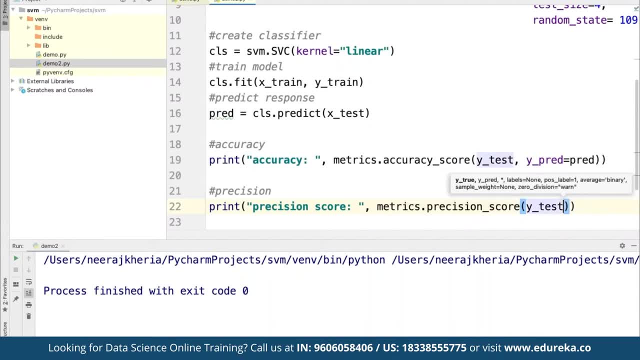 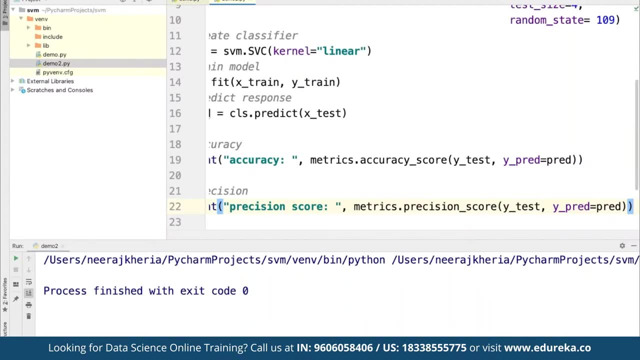 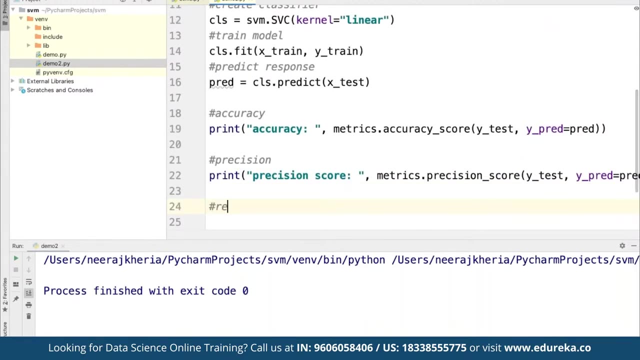 we are going to make use of y test and then we are going to make use of y prediction, all right. and then at the end, if you are simply going to recall the score and we are simply going to report, so here we can define for recall, we can print another statement for recall. we can define. 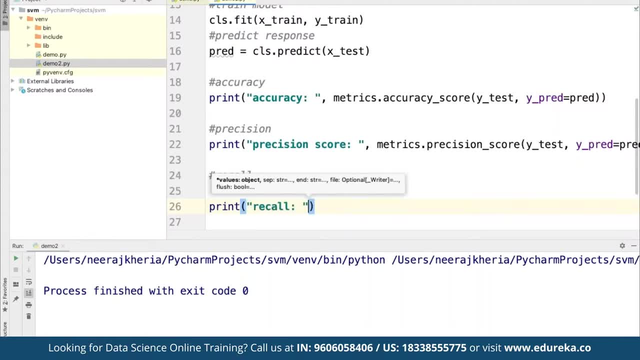 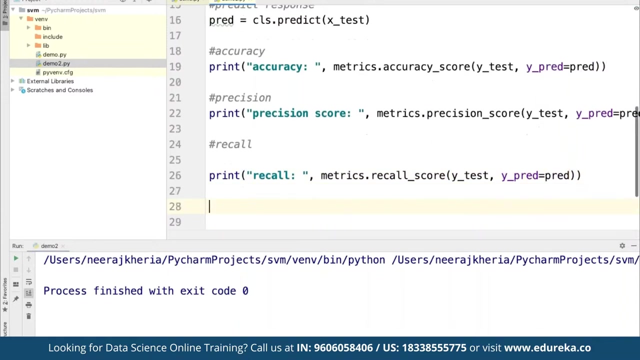 this one as recall, and here from save metrics dot recall score, and for here we can define y test and y prediction for the prediction that we are going to define. and then if you want to print all the metrics, so here we're going to find print matrix dot plus. 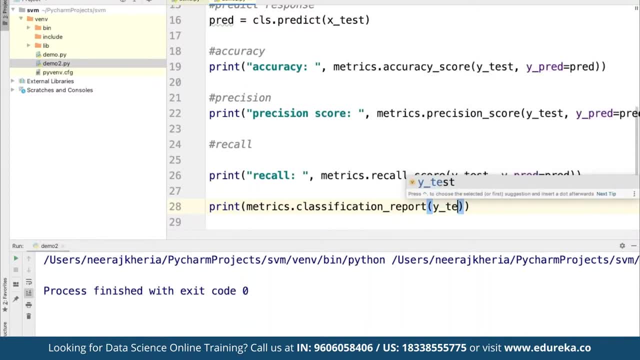 classification report, and for that we are going to make use of y test and y prediction, for prediction made all right. so here we had to find these, and now, once we have configured everything, so here we can simply run this up and we would be able to see the entire output which, once it has been defined, so now we can see, here we have the. 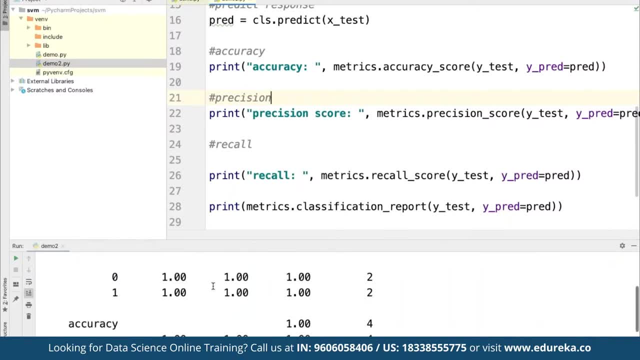 accuracy. here we have the precision score, the recall score that we had defined, and and then we define the accuracy based on whatever data we are going to work on. depending upon that we are simply define the current data set here. thank you so much for joining, guys, and have a.